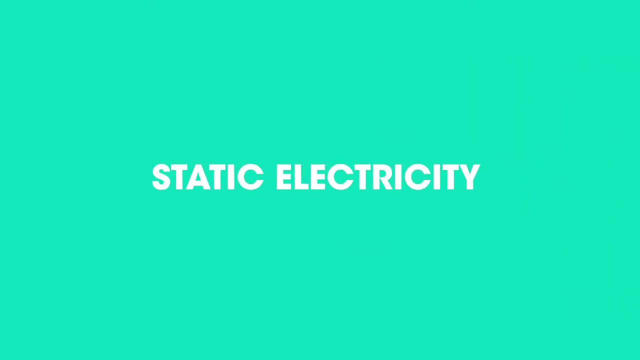 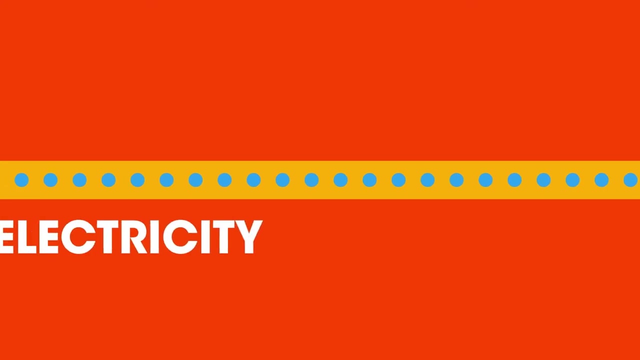 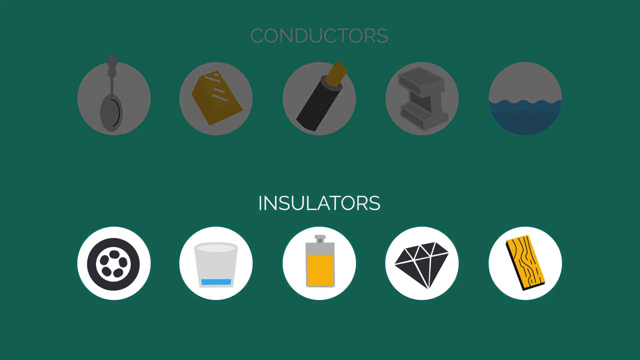 discovery, whereas the effects of static electricity were written about over 2,000 years ago in ancient Greece. As the name, static electricity suggests, it is static. it doesn't move. Metals allow the flow of electrons in current electricity, but here we are dealing with all the other materials that are not metals and are insulators, If two different. 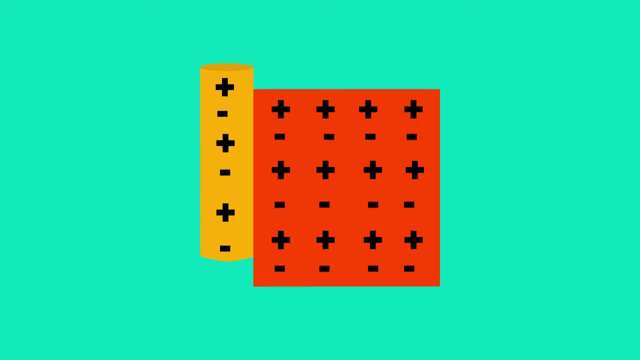 non-metal insulators — a cloth and a glass rod, for example — rub against each other, then both may become charged by friction. As they rub together, electrons may be removed from the surface of one and deposited on the surface of the other. Once there. 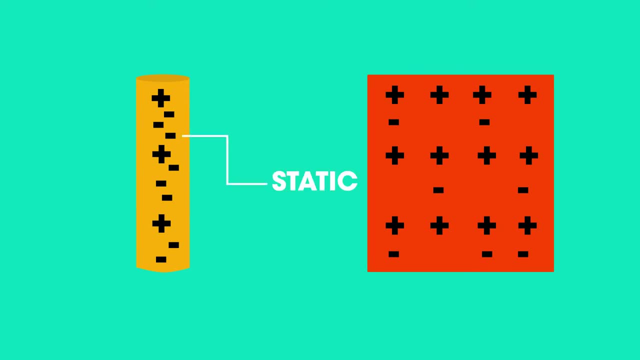 the electrons cannot move — they are static, Since all materials are naturally electrically neutral because they have an equal number of protons to electrons. This transfer of electrons leaves one material with less electrons and less negative charge than it had before, and the other material has more electrons, so one of the materials becomes positively charged and the other is negatively charged. 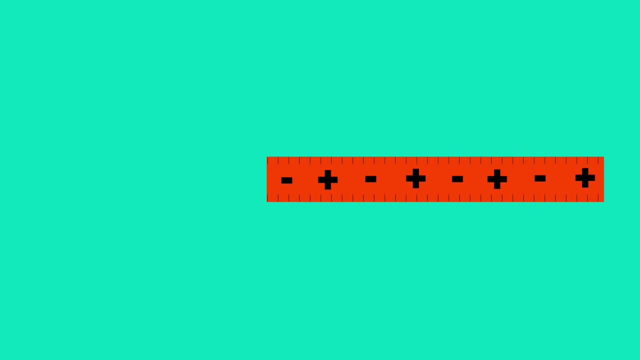 This can be seen when a plastic rod, such as a ruler, is rubbed with a soft cloth. Electrons may be transferred from the cloth to the ruler If two identical rulers are charged in this way and one is suspended in a simple cradle, as shown. 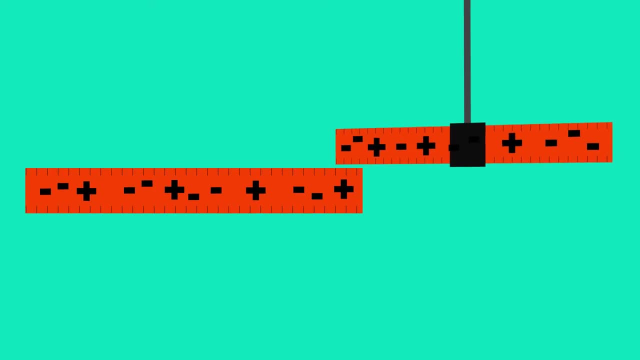 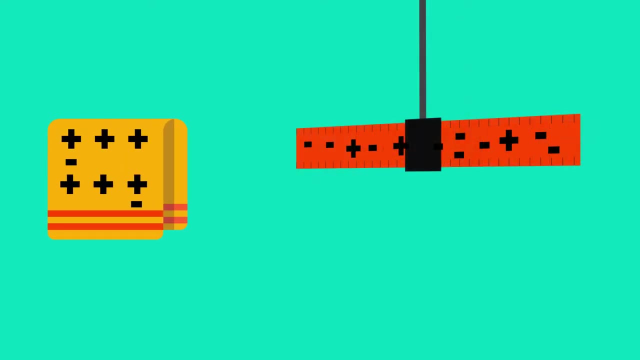 as the end of one ruler is brought closer to the other, repulsion is seen. as the suspended ruler turns, it is pushed away. Holding the cloth used for charging near to the ruler will attract it toward the cloth. This shows that there are two types of charge: positive and negative. 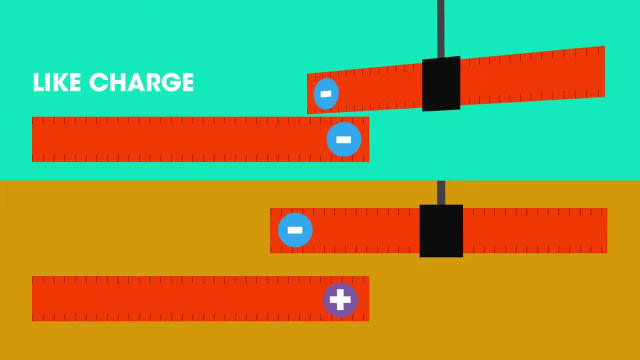 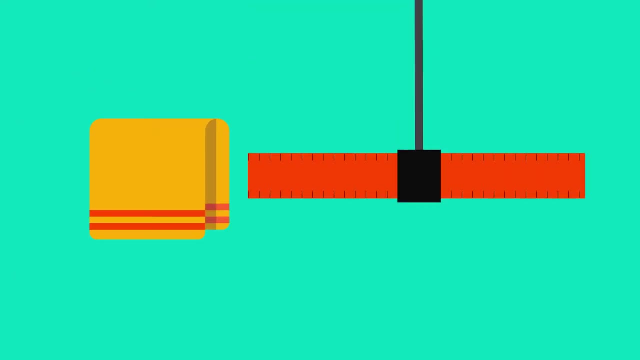 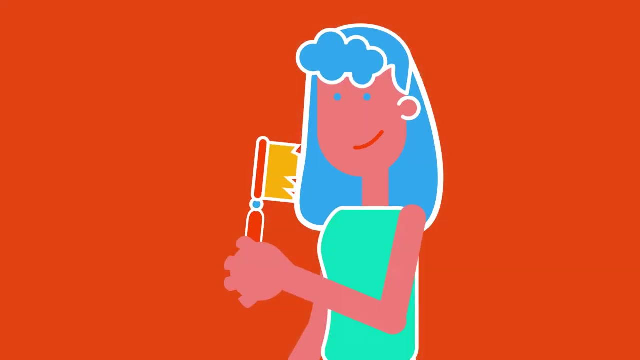 So alike charges repel or push each other away, whereas opposite charges attract each other or move towards each other. Which material becomes positive or negative depends on the identity of each. This happens when you brush your hair. The brush and the hair take on opposite charges and so become attracted to each other.